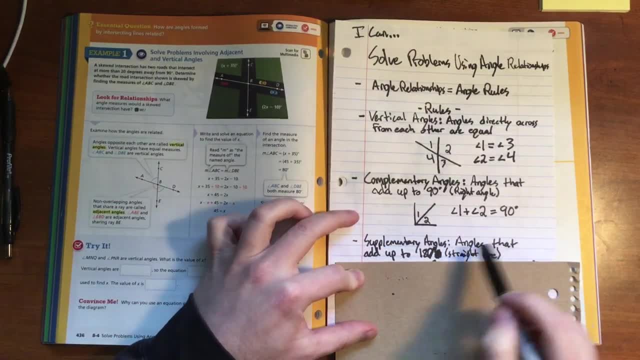 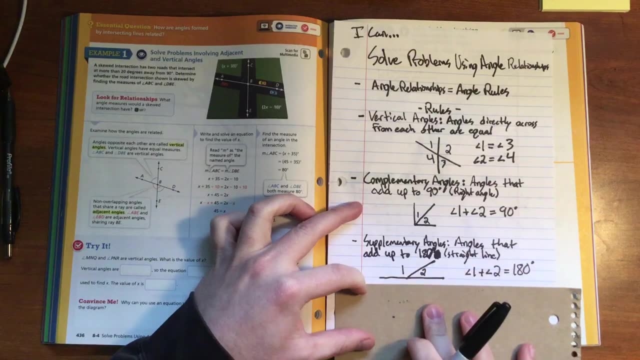 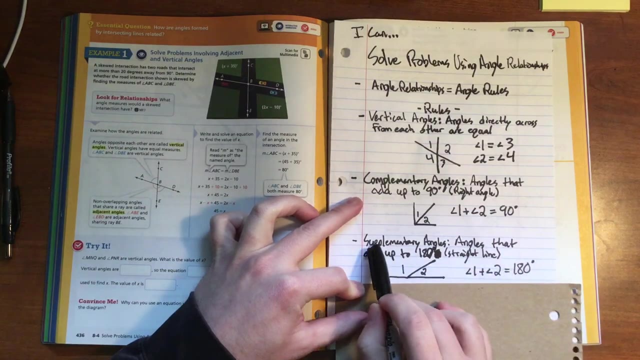 we have supplementary angles. These are angles that add up to 180 degrees or they add together to make a straight line. So if we look at these right here, angle one and angle two add up to 180 degrees, so they are supplementary angles. So if you see, 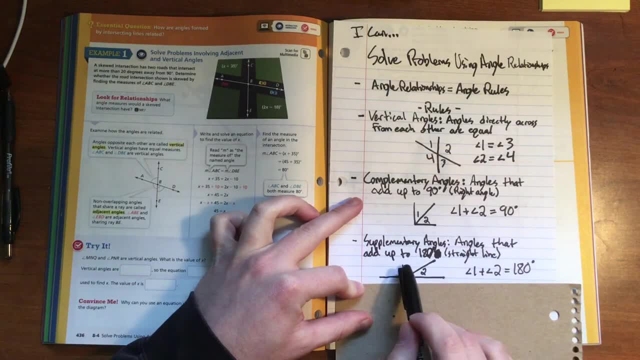 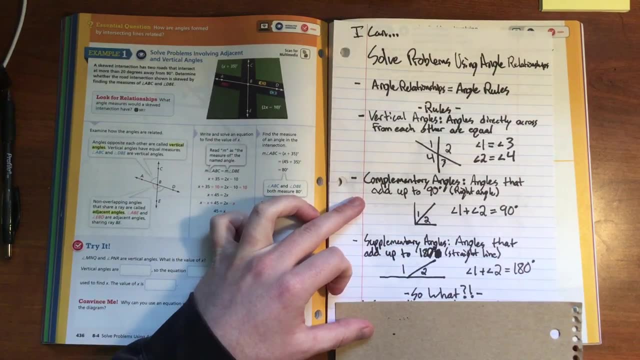 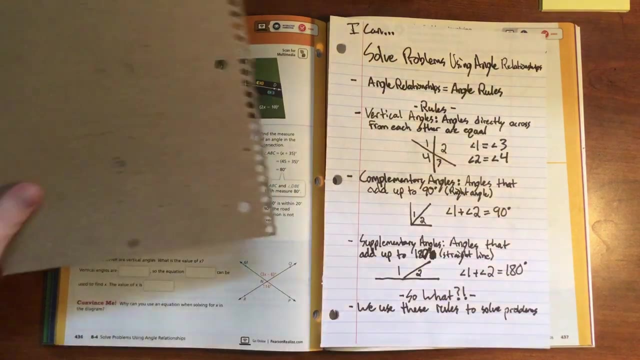 two angles that sit on a flat line, then they would add up to 180 degrees, making them supplementary angles. All right, so what? Why do we need to know these? Well, we're going to use these rules to solve problems. Let's look at our first example. This says angle MNQ. 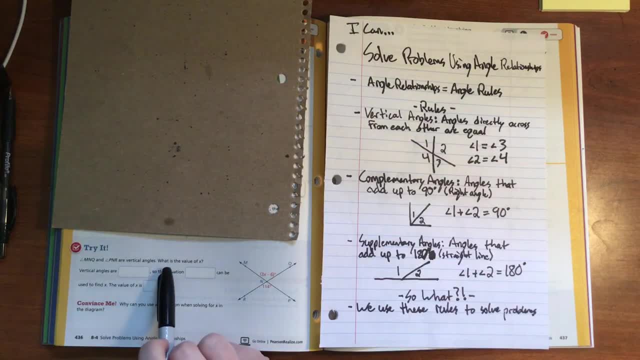 and angle PNR are vertical angles. What is the value of x? Well, it tells us they're vertical angles. so we know these two angles are equal, All right. angle MNQ: it says it's 3x minus 6. 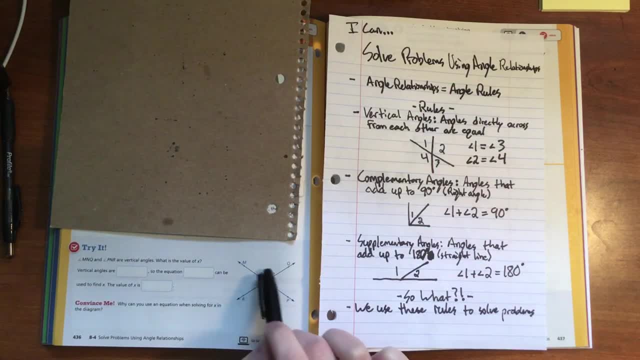 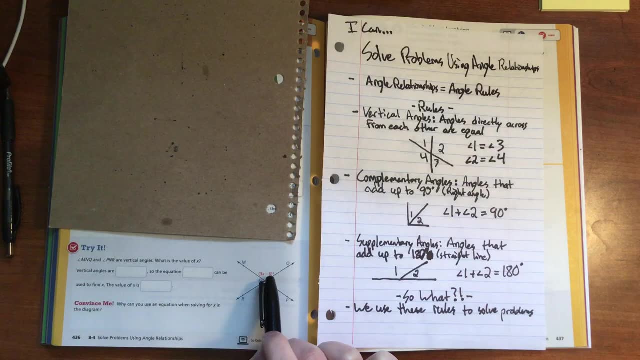 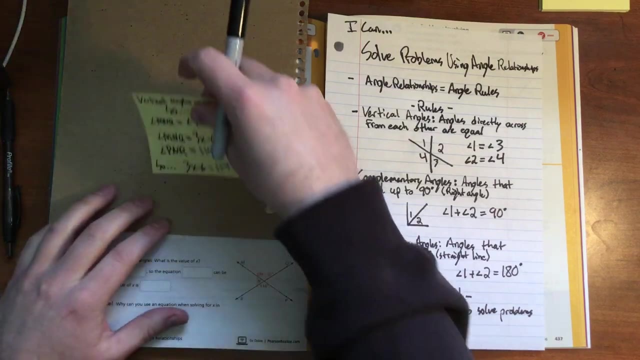 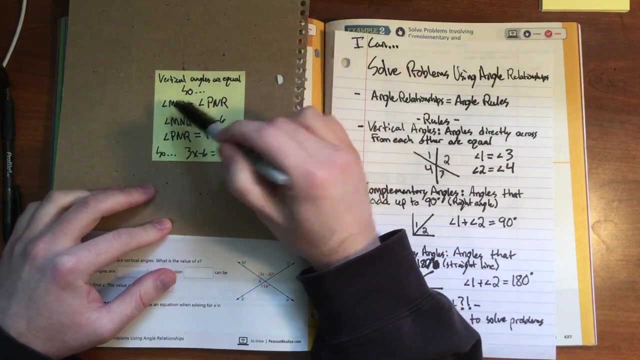 degrees. So this angle, they're not giving us the exact degree, but they're telling us it's equal to 3x minus 6.. Okay, angle PNR is 114 degrees, So vertical angles are equal. so that means, since these two are vertical angles, 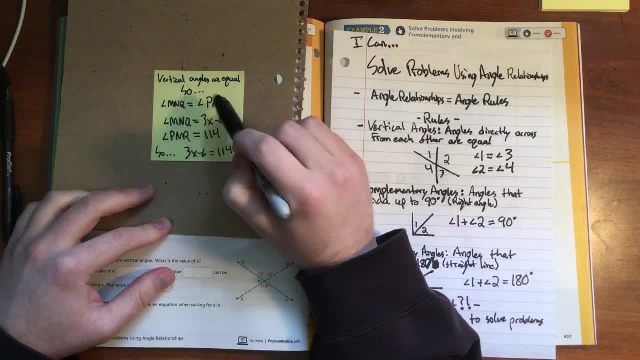 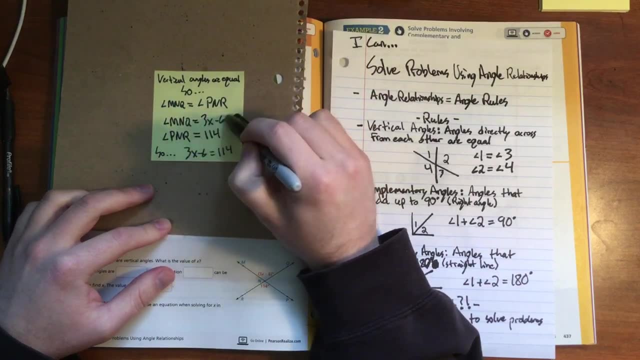 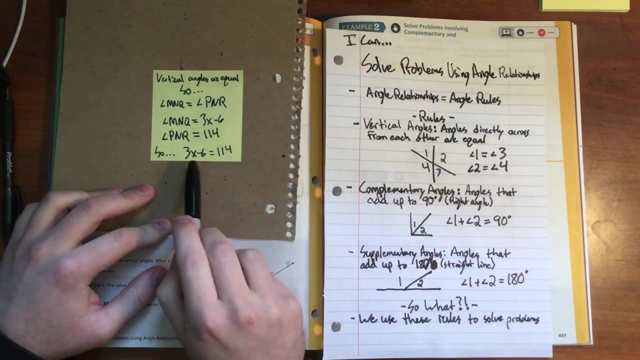 then they are equal. So angle MNQ is equal to angle PNR. Here's the other information we know: MNQ is equal to 3x minus 6, and PNR is equal to 114.. So that means that 3x minus 6,. 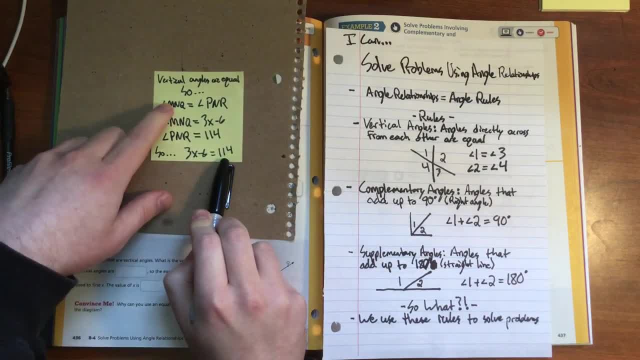 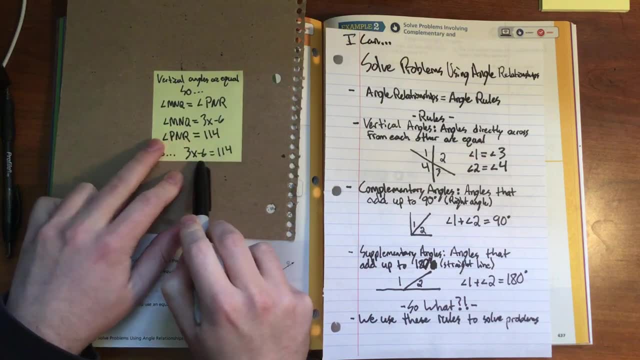 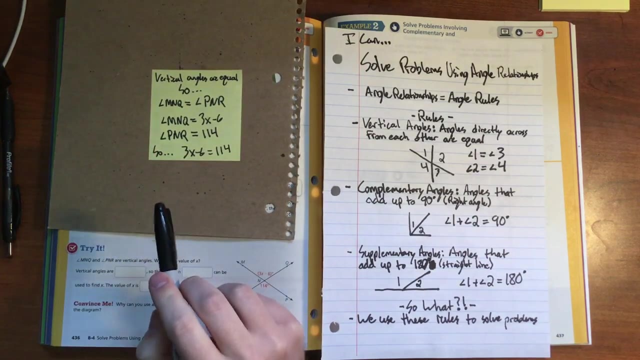 is equal to 114.. Again, because MNQ equals 3x minus 6, PNR equals 14, so that means that these two things are equal. Now this looks like just a regular old equation that we can solve, So this: 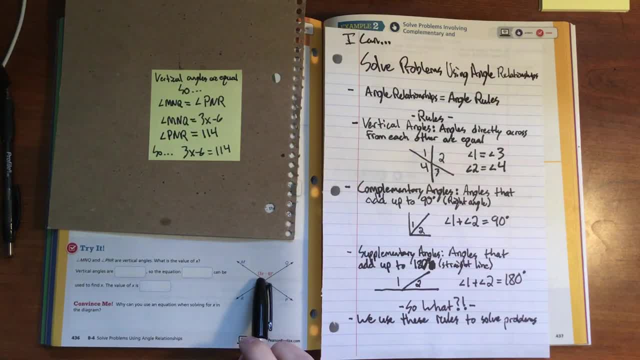 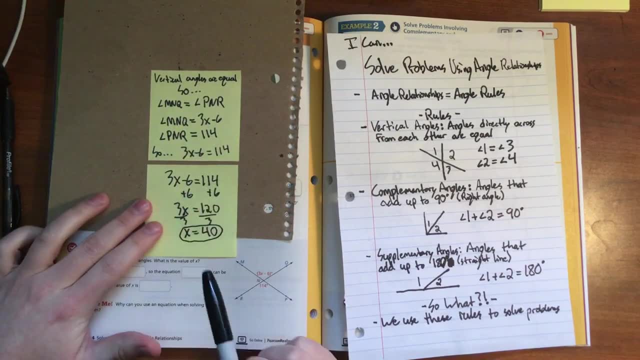 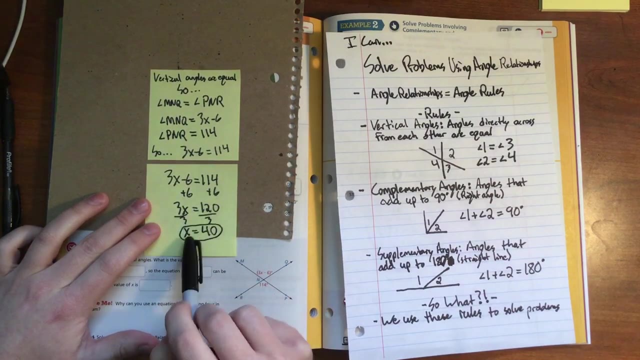 question down here is wanting to know what is the value of x. Well, we've set up an equation, so now all we have to do is solve for x. 3x minus 6 equals 114,. we add 6 to both sides to get rid of this. then we divide by 3 to get rid of that and we get x. 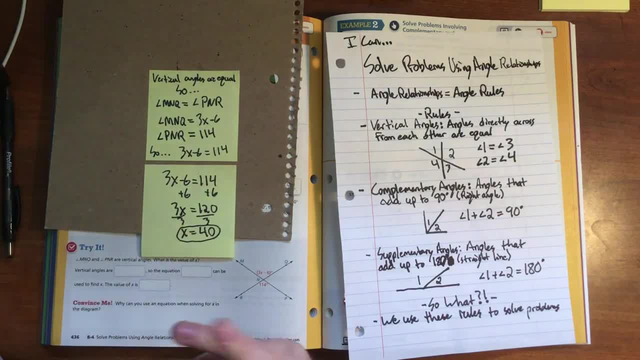 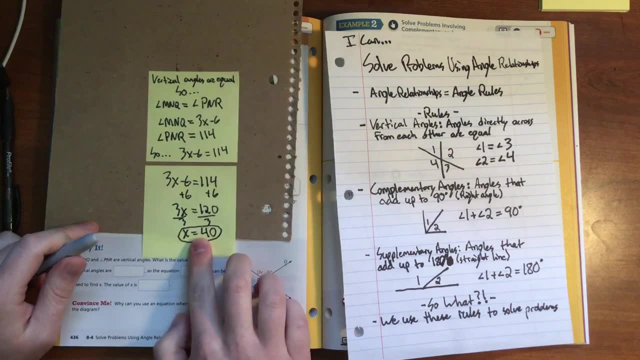 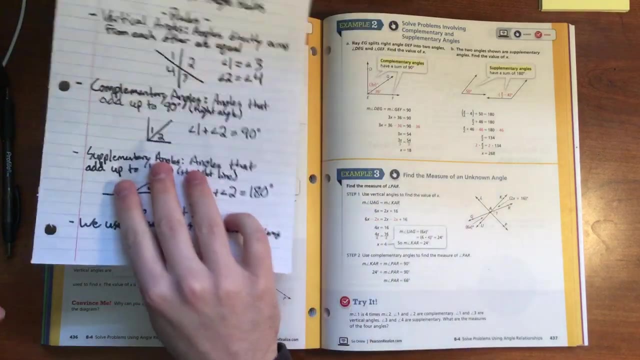 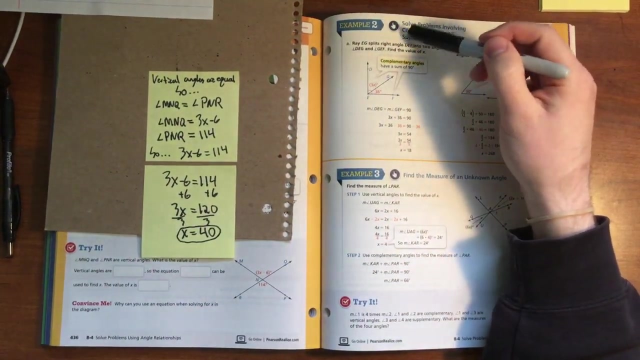 equals 40.. Okay, so we used the angle rule of vertical angles to set up an equation. then we solved the equation to find the missing variable in the diagram. Okay, let's look at another couple examples. Ray, EG, EG, EG fits right angle DEF into two angles. so it's telling us DEF is a right angle, So that gives. 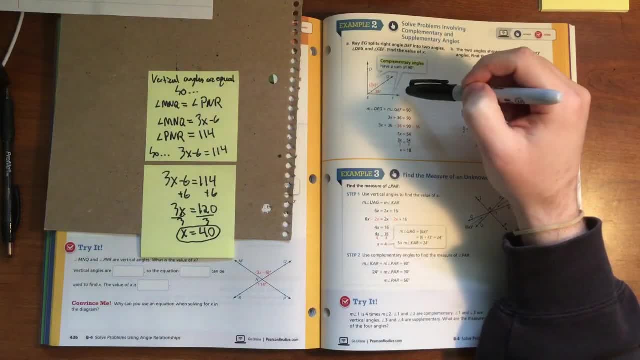 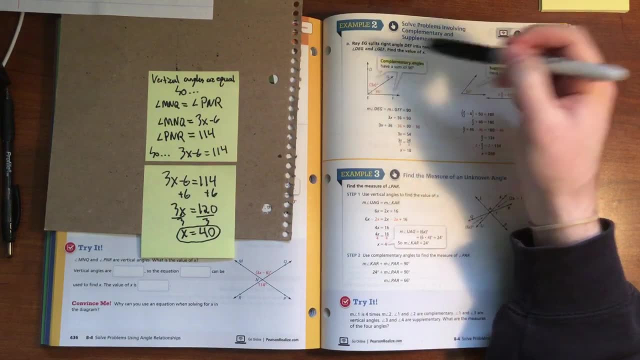 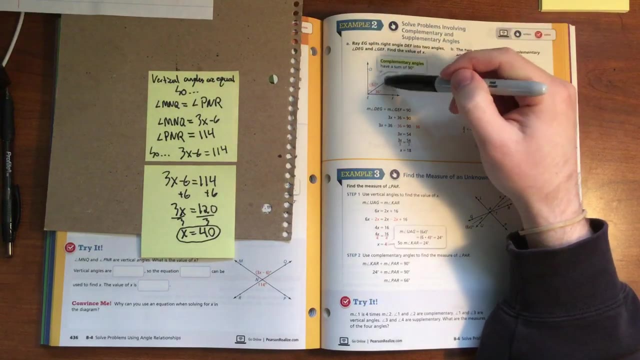 us two more angles: DEG and GEF. It says: find the value of x. Well, we don't know what x equals. that's why we're looking for it. but we do know these two angles right here are complementary angles. so that means they add up to 90 degrees. So this angle plus this angle equals 90 degrees. 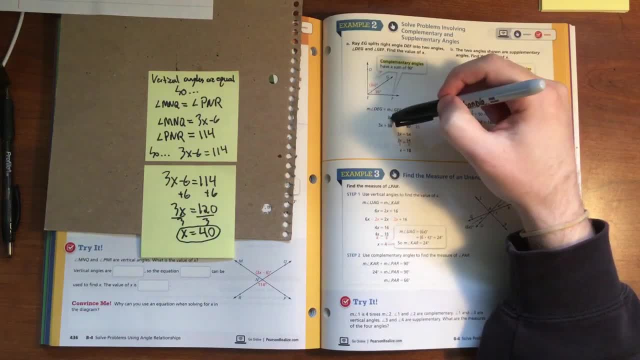 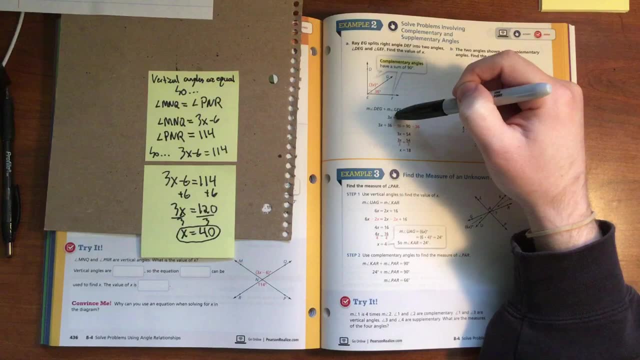 DEG equals 3x, which we have written right here. City F equals 36 degrees, DEF is 36, so if we now, if we add them together, it should give us 90 degrees. But then, right there, we need T-sides. 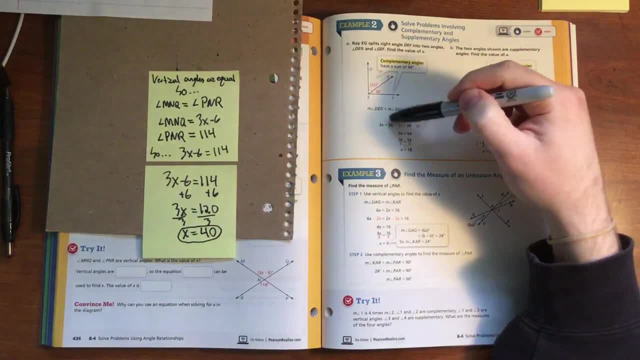 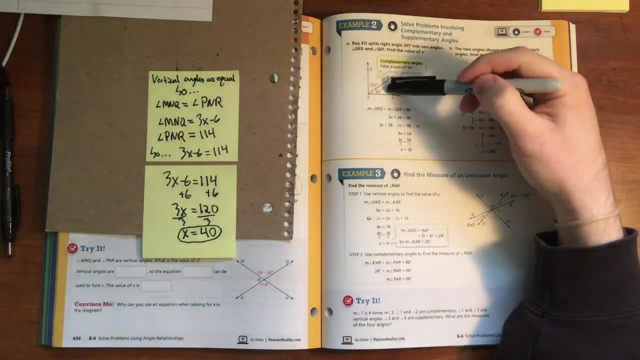 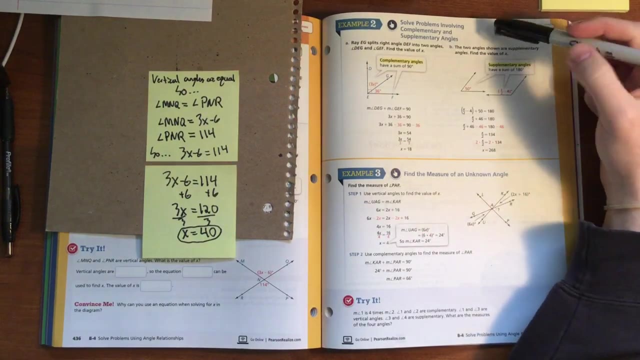 of the equation that we can solve. so we go through and get rid of everything around T and we get x equals eighteen. and again we are able to find that because these two is a complimentary, which means when I addiab them together they equal 90 degrees. Over here it tells us the two angles shown are supplementary angles, So that 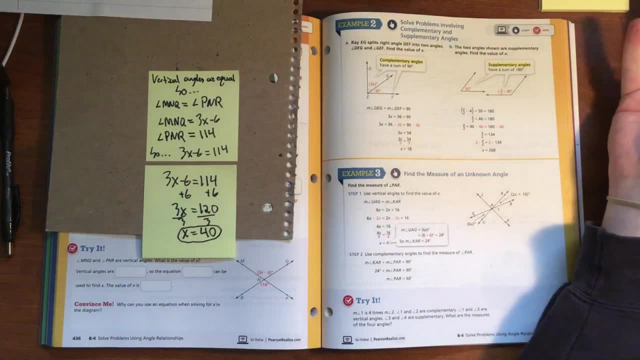 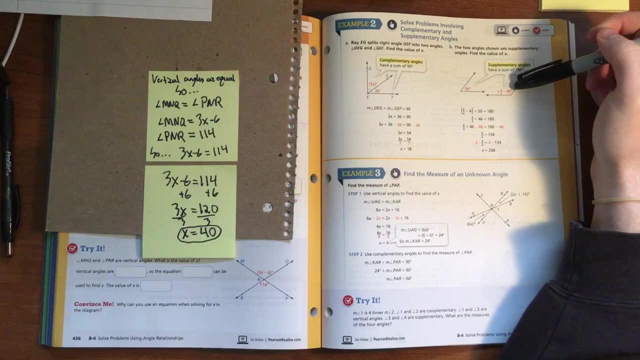 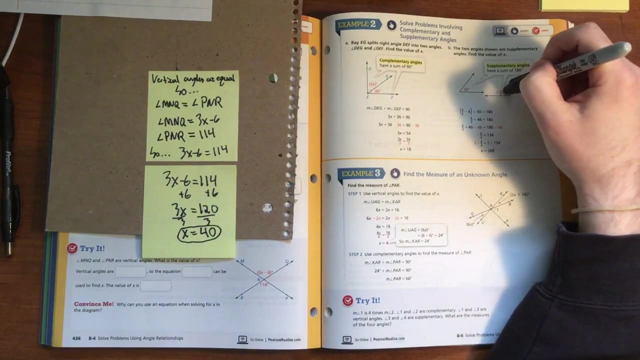 tells us that if I were to put them together, they would make a straight line or they would add up to 180 degrees. So this angle is 50 degrees and this angle is the quantity of x over 2 minus 4.. So if I add these together, they're equal to 180 degrees, which, as you can see right here, is what they did. 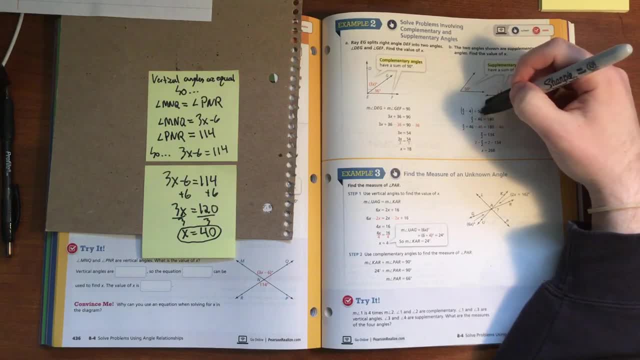 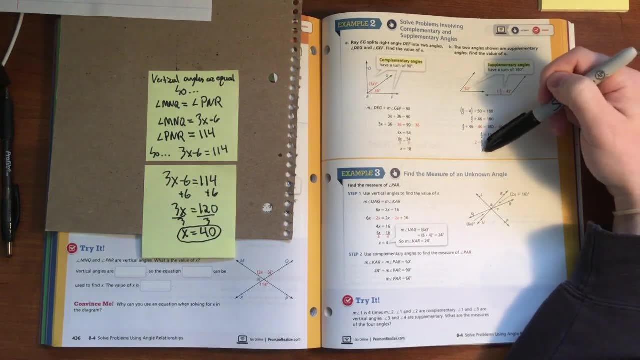 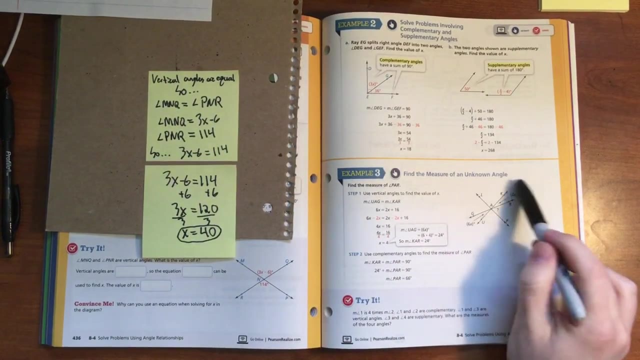 So all they did is simplified right here and then solved for x. So they go through, they get rid of everything around x, and they found that x equals 268 degrees. Okay, lastly, we're going to get diagrams that look a little bit more complicated, and so we'll have to be 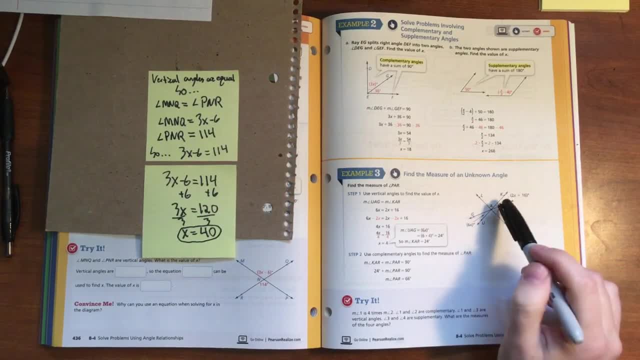 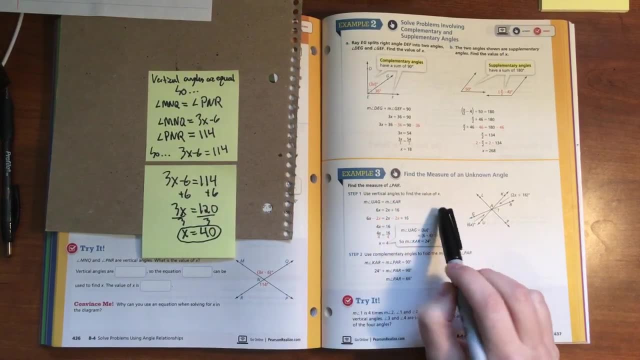 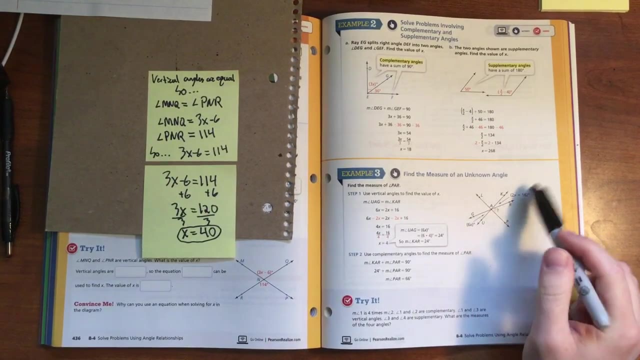 really good about knowing our angle rules and being able to look at just the angles that they're talking about. This one says: use vertical angles to find the value of x. Well, right here it tells us. this angle, UAG, is 6x. and then this angle, KAR, is equal to the quantity of 2x plus 16.. 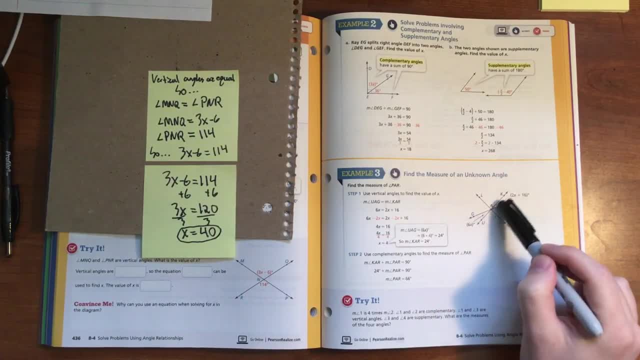 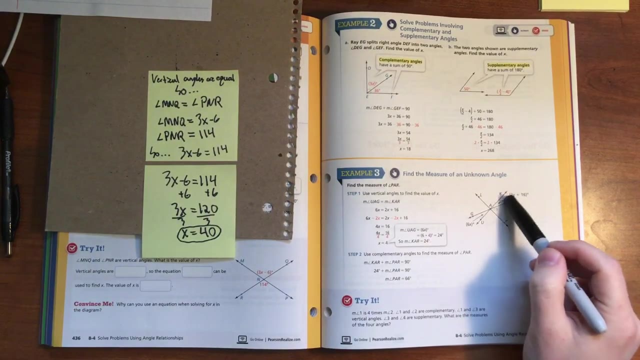 They are angles that are directly facing each other. They're opposite each other. Okay, they're directly across from each other. so that tells us, since they're vertical angles, that 6x or this angle is equal to the quantity of 2x plus 16, which is this angle. So we can use that to set up an. 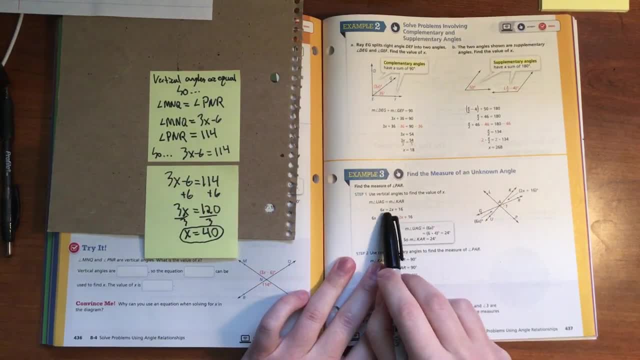 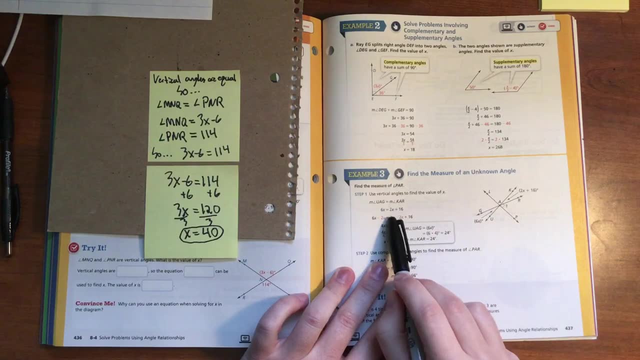 equation: 6x, or the first angle, is equal to 2x plus 16, which is the second angle. Then we just go through and simplify. So they subtracted 2x from both sides to get 4x equals 16,. 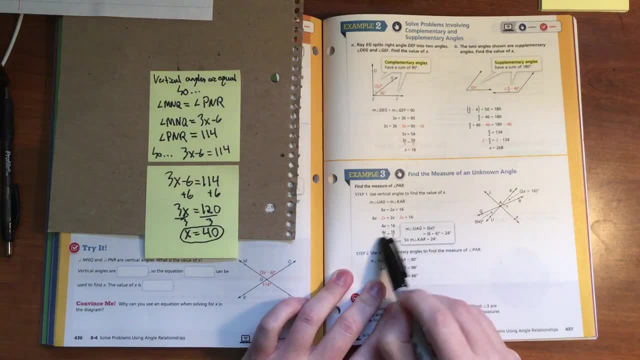 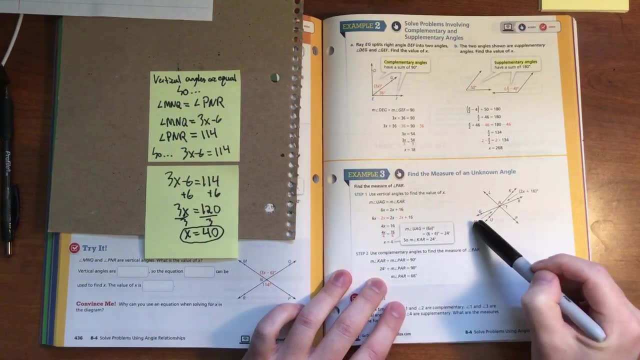 divided by 4 on both sides, and we get x equals 4.. Again, we use the property of vertical angles, which are angles that face each other, to show that 6x is equal to 2x plus 16. We set up the 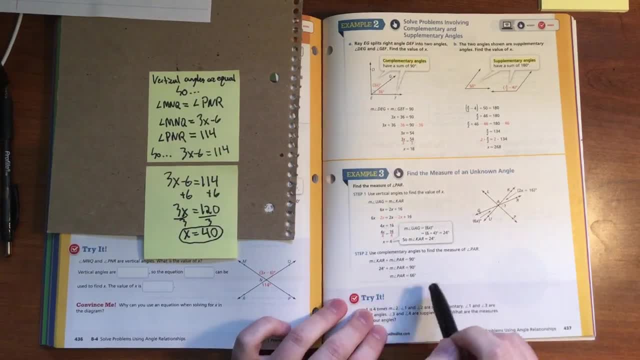 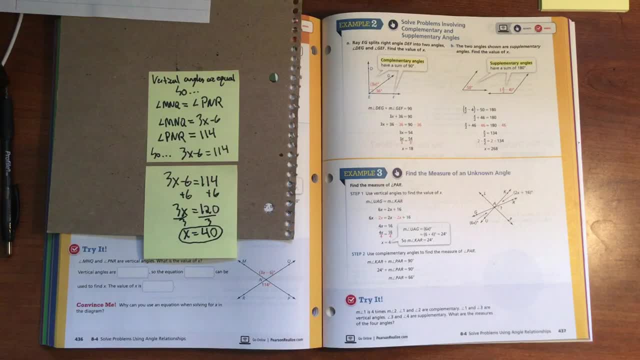 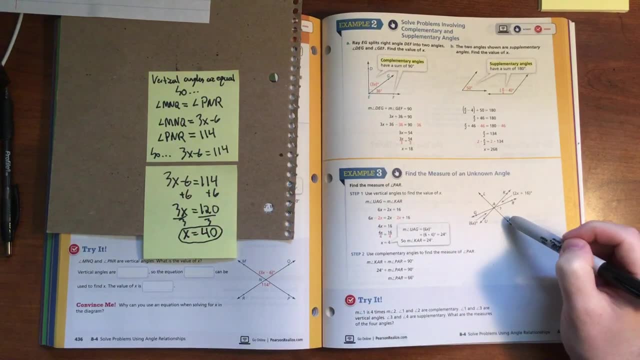 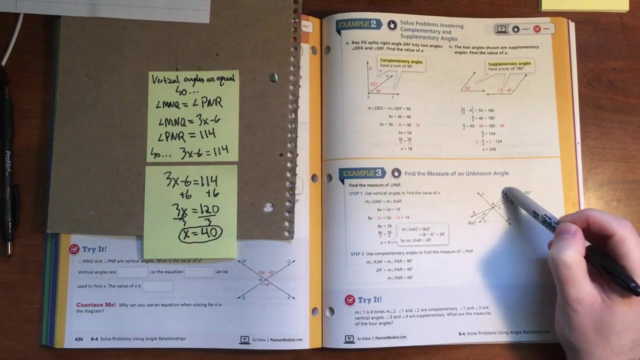 P-A-R- Okay, if you recall, complementary angles add up to 90 degrees. So P-A-R is the angle right here. P-A-R- All right, it makes a complementary angle with K-A-R. See how they have it marked. 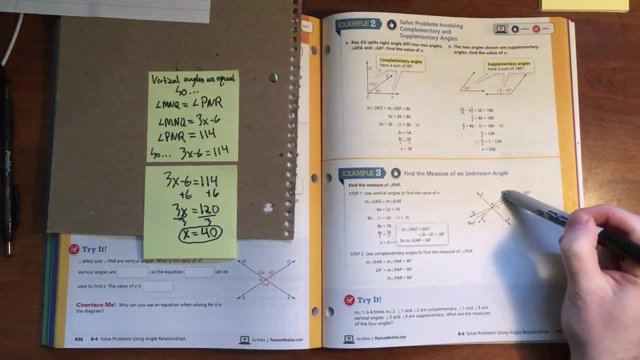 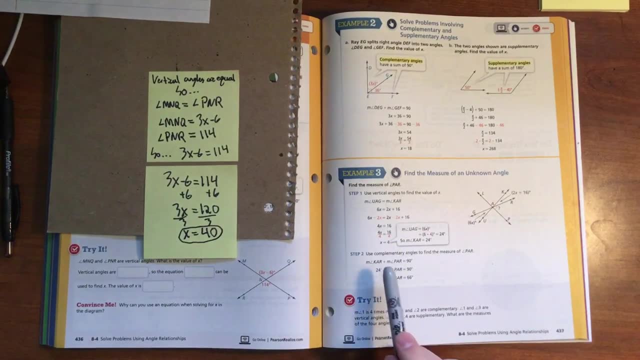 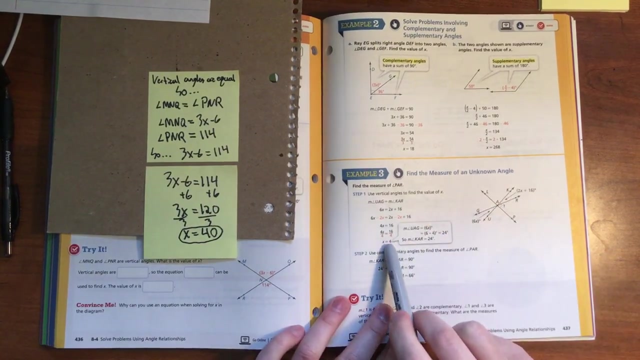 right here that this is 90 degrees, So that means this angle plus this angle equals 90 degrees. Okay, so down here the first angle that we know. all right, because we can figure that out now using X right here. So they used X to figure out that K-A-R is equal to 24 degrees, So they 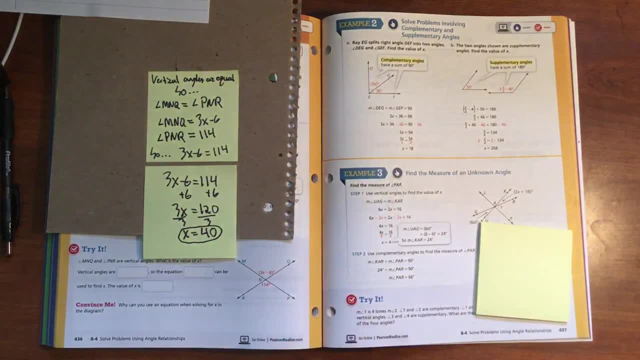 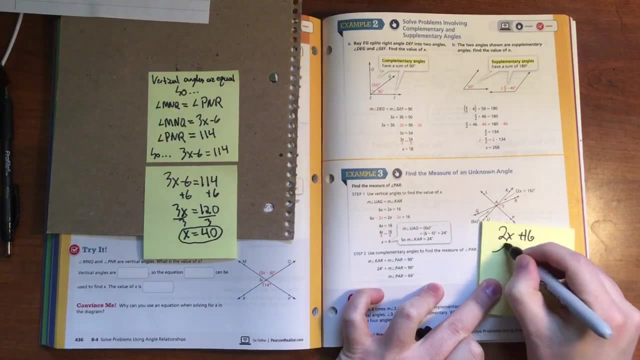 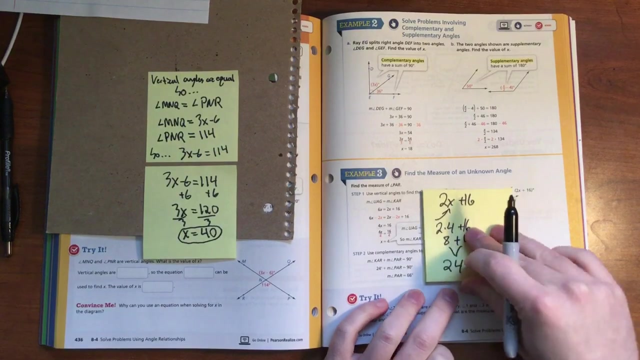 plugged in 4 for X, So they found X equals 4.. So instead of 2X plus 16, they subbed in 4 for X, So this is now 2 times 4. Plus 16. So they get 8 plus 16 equals 24.. We can now use that information. 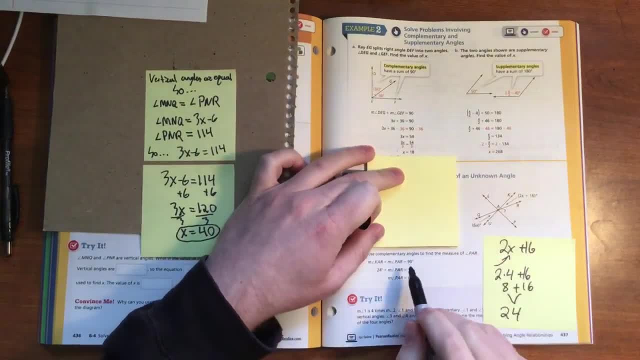 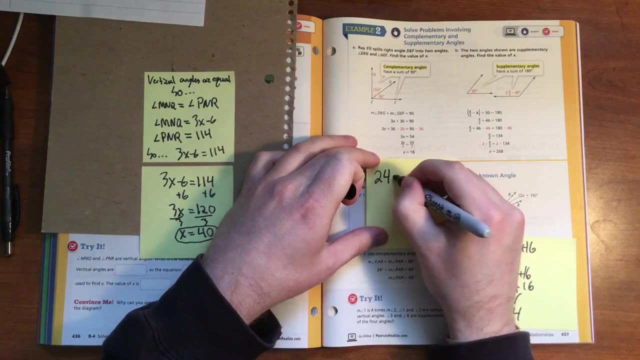 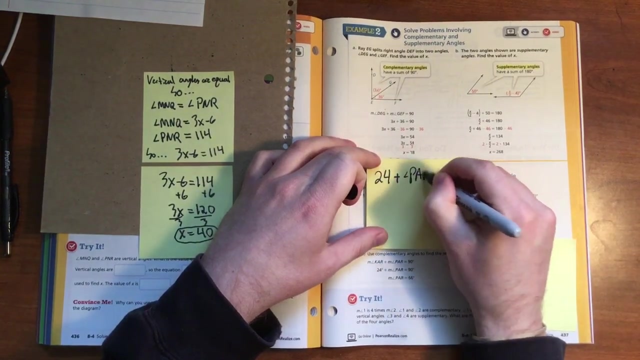 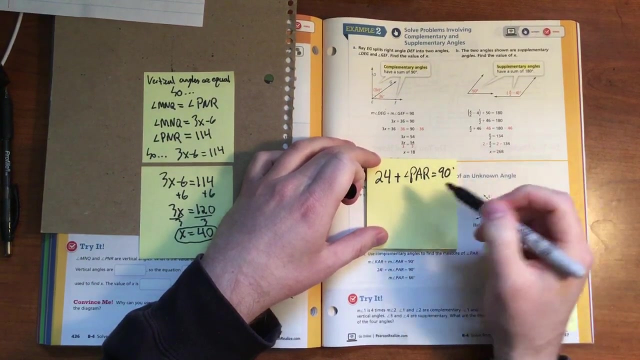 to find P-A-R. Okay, so we know this angle, which is 24, plus whatever P-A-R is, has to equal 90 degrees. Since they're complementary, they add up to 90 degrees. All right, we can substitute a variable. 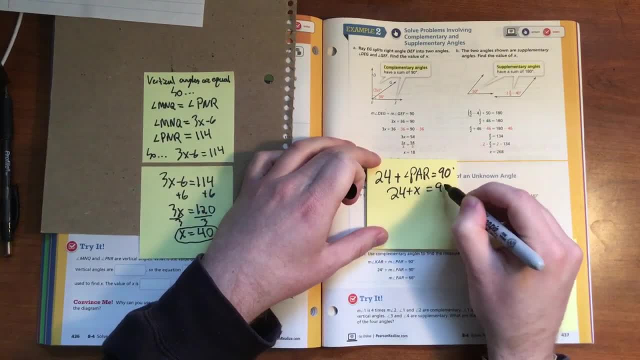 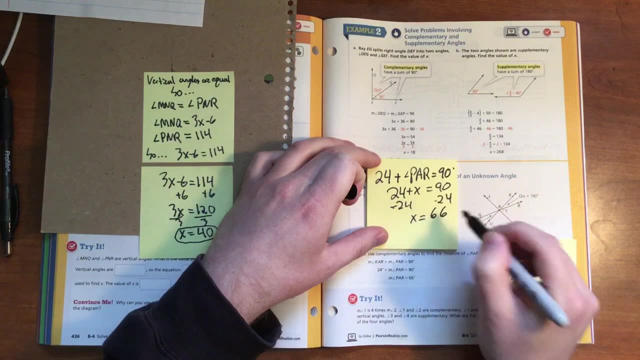 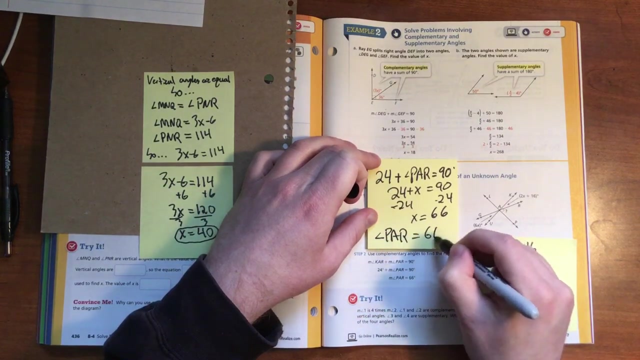 in here, if you'd like. 24 plus X equals 90.. Subtract 24 from both sides and you should get X equals 66, which means that angle P-A-R is 66 degrees. Okay, so again the whole process that. 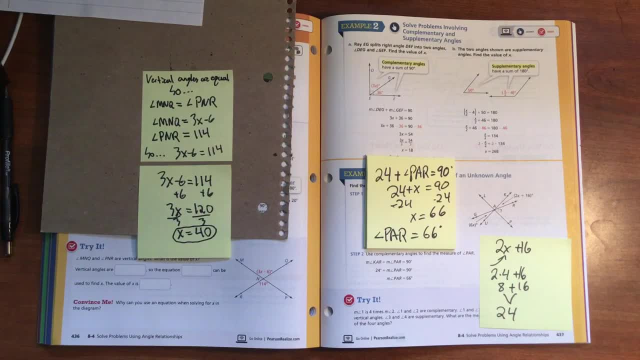 we're using to find P-A-R is to find P-A-R, So we can substitute a variable in here if you'd like. So what we're going to do today is using our angle rules of vertical angles, complementary angles and 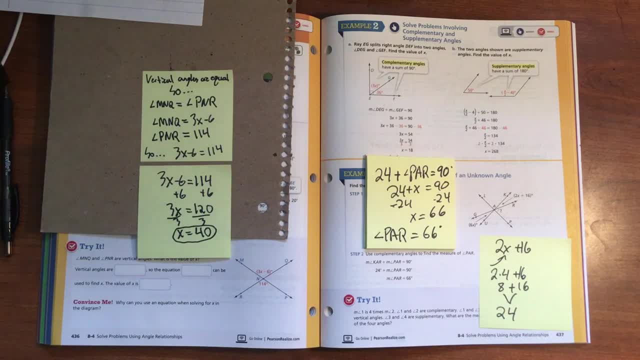 supplementary angles, to find new information, to set up equations, to figure out what missing angles and missing variables are equal to. If you guys have any questions or need any help, as always feel free to email me or you can write questions down and bring them up during conferences. All right, I'll.